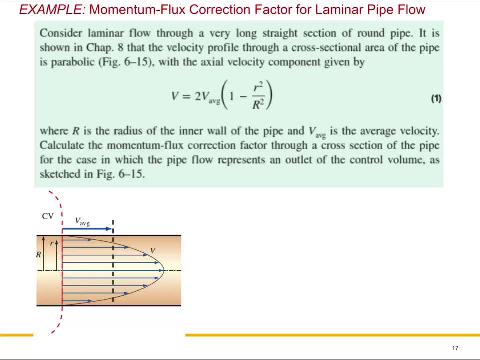 Plex correction factor for Levenor pipe flow. So this is the schematic. You can see this is the pipe cross-sectional view. This is the radius R. Here you can see it is a fully developed flow profile. So this dotted line is showing the control volume. This black dotted line, this is the average velocity. So you already know why we usually use the average velocity for this sort of problems. So in this question it says consider a laminar flow through a very long straight section of a round pipe. And the velocity profile is like this. So here this is the average velocity. You can see this average velocity. R is this radius, radius of the pipe. 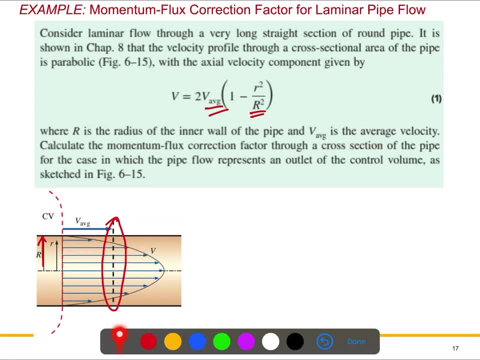 So B is the average velocity. So we need to calculate the momentum Plex corrections factor. So we need to calculate the momentum Plex corrections factor. We usually define this is beta, right? We know from the theories. And it also says, you can see here, calculate the momentum Plex corrections factor through a cross-section of the pipe. 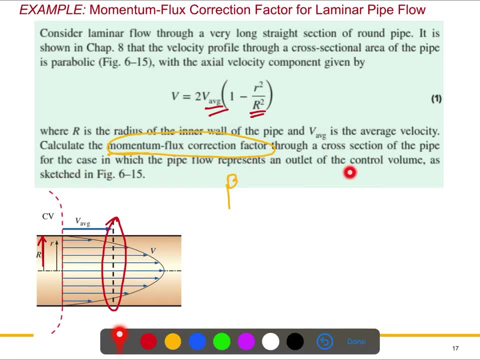 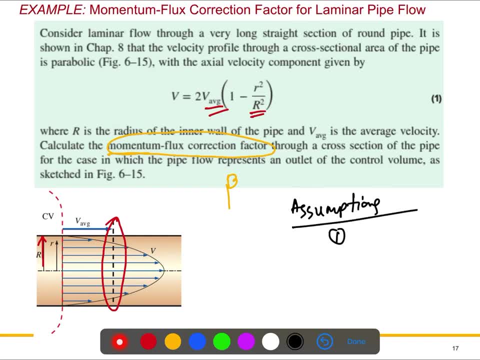 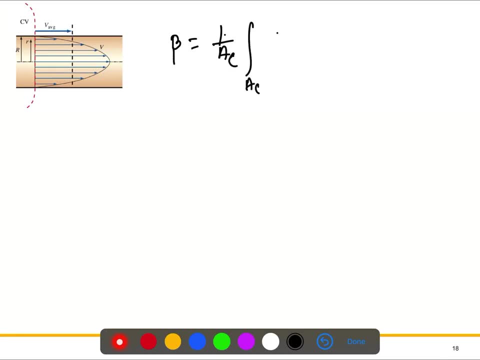 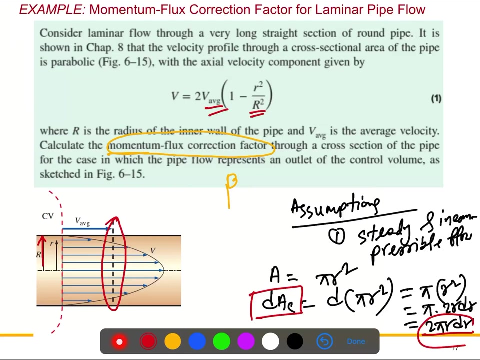 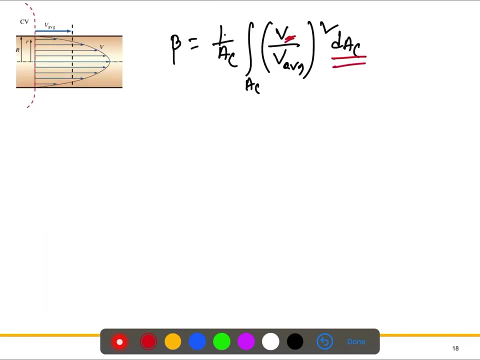 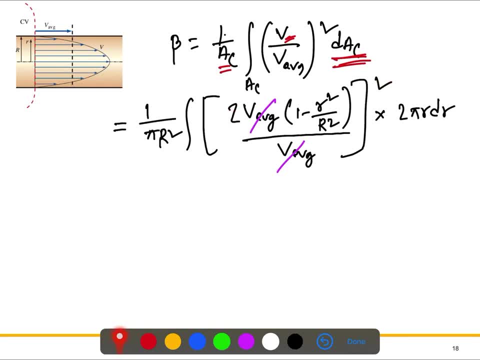 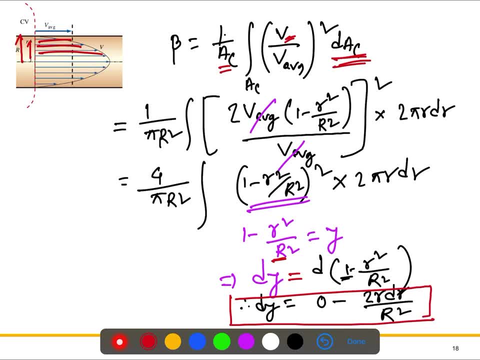 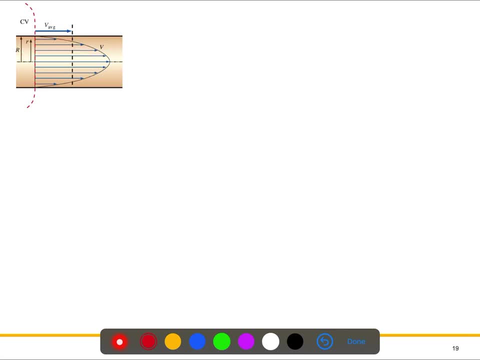 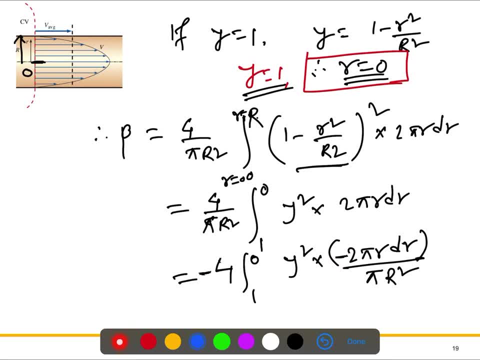 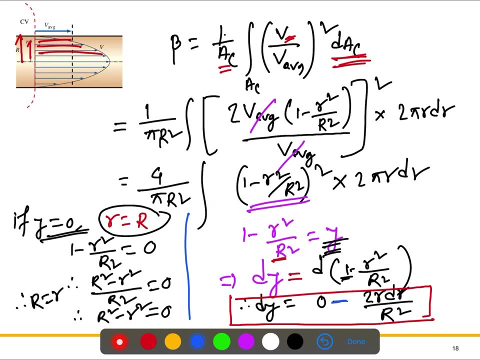 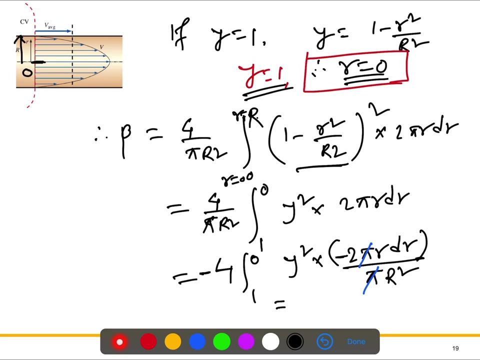